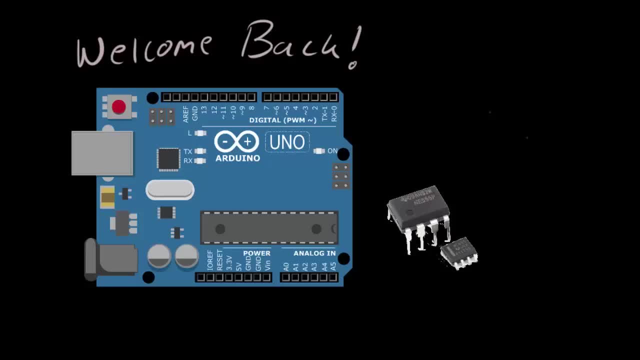 on them, but they're really nice to know about, and every electronics hobbyist should have some form of a microcontroller that they can just program and experiment with. So what in the world is a microcontroller? Well, as you can see on the screen, I'm sure most of you have heard of 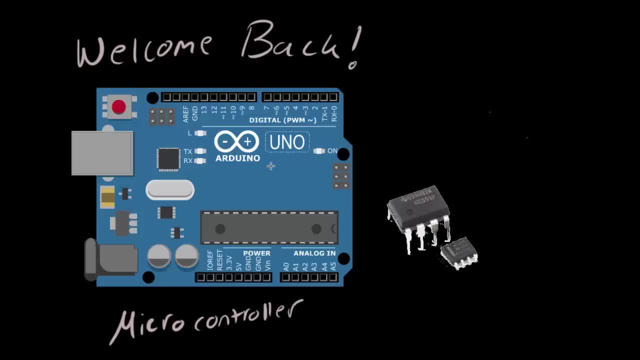 Arduino, and Arduino might be one of the most popular forms of a beginner microcontroller out there. that's programmable And a microcontroller is essentially just a little tiny computer. It can have obviously a CPU and memory and everything like that on an IC. 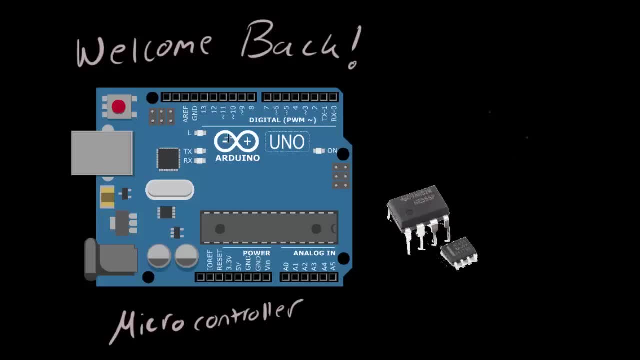 on an integrated circuit chip. So in the case of the classic Arduino Uno, it comes in a board that looks something like this: It simply has this microcontroller chip on it, along with other devices on the board to make the microcontroller work. as well as you know, pin. 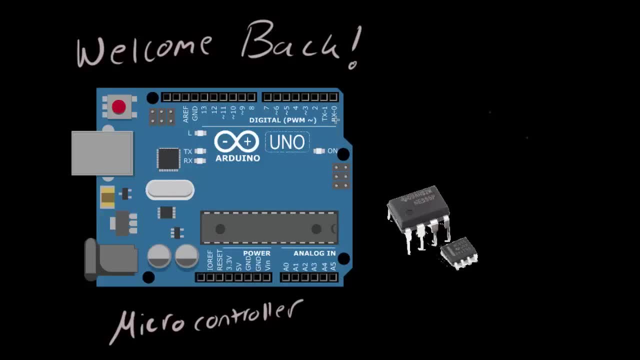 outputs down here and pin inputs and stuff like that. And this classic Arduino chip can simply be plugged into your computer, you program it and you upload your code to the chip and it will essentially run and you can control stuff via these input and output pins here. But there's 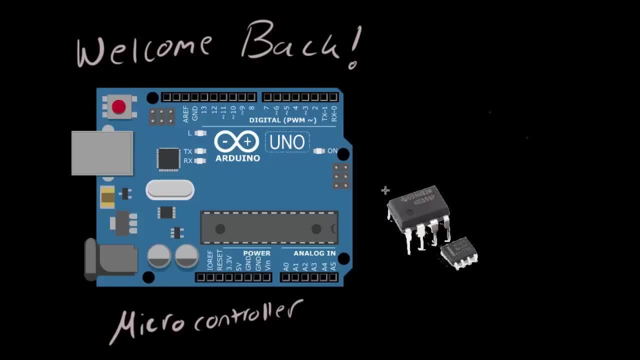 loads and loads of different microcontrollers. By all means, Arduino is not the only type, but they're one of the more common ones for this level of electronics work. Another microcontroller that I've used on many, many different projects is the ATtiny85.. The ATtiny85 is kind of based off of 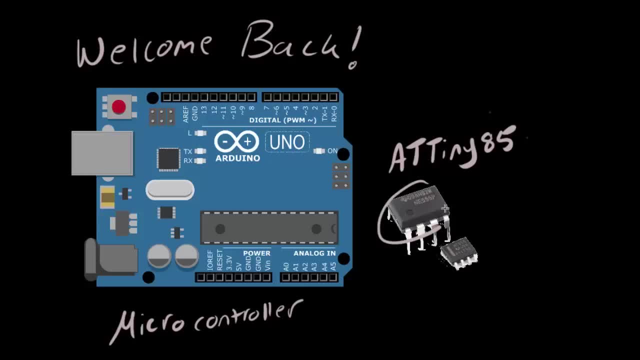 Arduino. It's much smaller. It comes in an 8-pin chip, Kind of like the triple 5 timer. it's just an 8 pin chip. You're able to program and upload code to it and use just a couple of input and output pins to accomplish a few tasks. 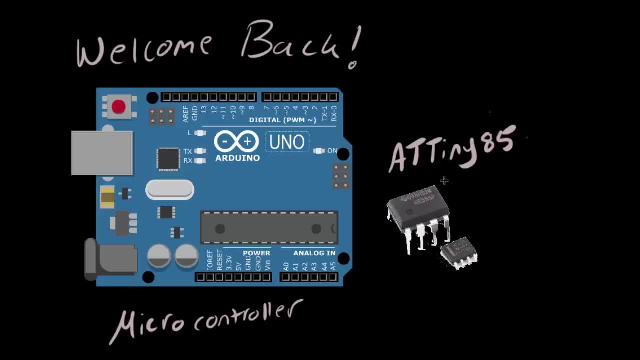 So microcontrollers are extremely useful and pretty common in many electronics hobbyist projects. Of course, we're not going to be using a microcontroller necessarily in our own 8-bit computer, though we might very well use it to debug stuff and make our lives a. 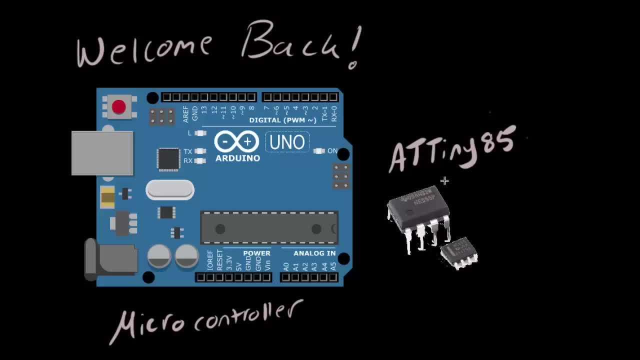 little bit easier while we develop it. But either way you should know how to program a microcontroller, because if you can't program a microcontroller like an Arduino in a higher level programming language, then it's going to be really difficult to describe what our 8-bit computer is going to do. 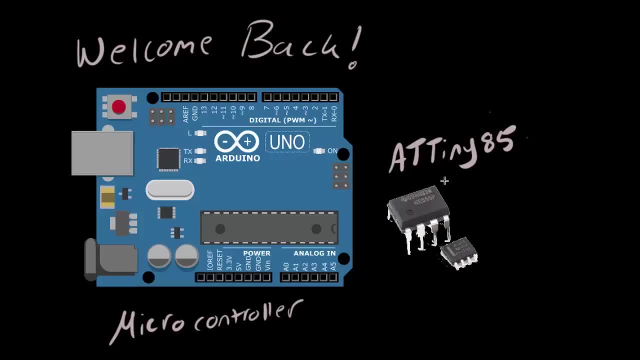 in a low-level assembly and opcode language. So, again, if you haven't gotten into these already, I highly recommend getting one. and just. there's loads of tutorials and articles online about these guys and how they can be used for many different projects. So, without further ado, let me get out. 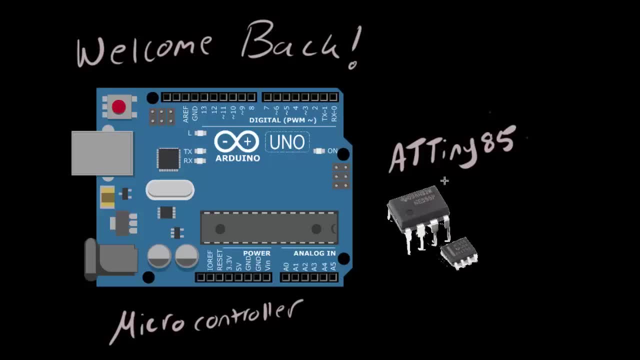 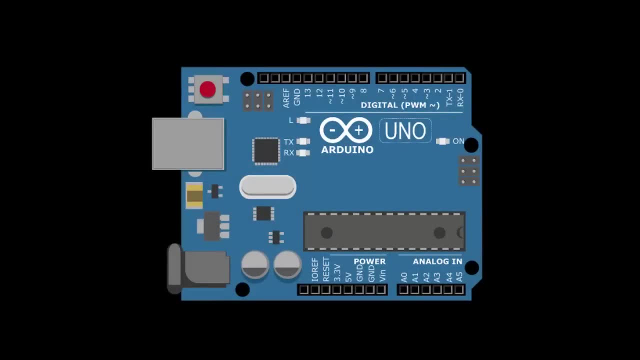 my Arduino Uno board and let's just program something really simple on it to see the basics of microcontroller programming. So let's talk a little bit about what we see on the Arduino Uno board here. Over here we have a USB port. Now this USB port functions as two things It can provide. 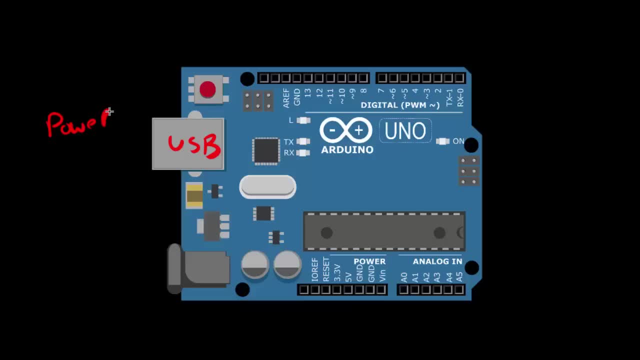 power to the board. so you can power this Arduino Uno board from your computer or from a USB port, And it also, of course, allows you to program the board. It allows you to upload the code to the Arduino board from your computer And the other way to power the board. 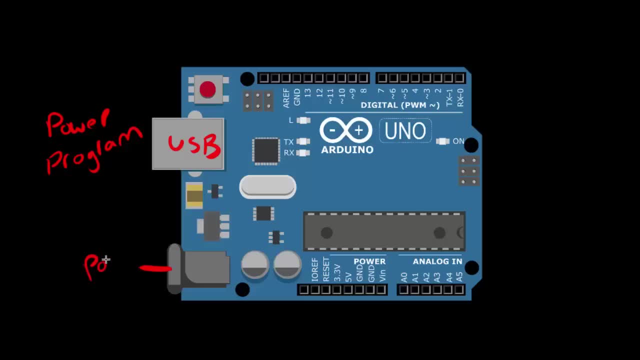 is through this port right down here. This can supply power to the board separately. That way, if you're done programming your board and you're done testing and you actually want to maybe sell this to someone inside of a product, then you would just power the board through this power. 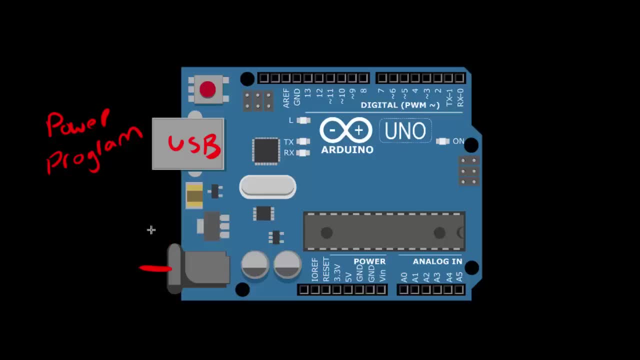 port down here. Now we're not going to be using this because we're going to be connected via a USB connection to our computer, Which is both going to power it and allow us to program it, So that USB connection is going to go to our 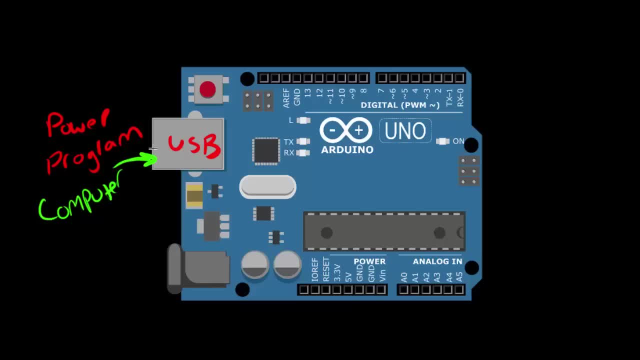 computer. So our computer is going to be connected through here. So now that the Uno board is powered up and we're connected, let's take a look at some of the power options that it supplies us with these output pins. down here We can see that it supplies two ground pins so we're able to connect to ground. 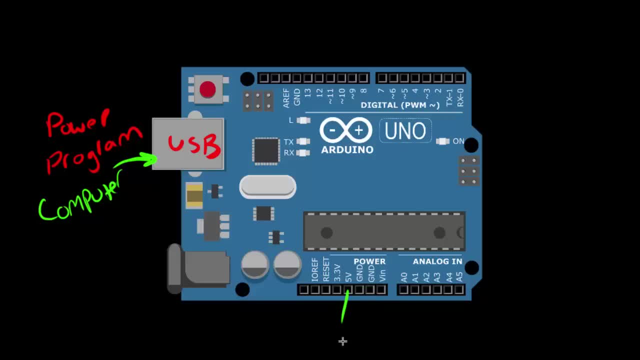 via these two pins here, And it also gives us a 5 volt output pin and a 3.3 volt output pin, So we can use those pins for powering our board. So we're going to go ahead and connect this to our computer. 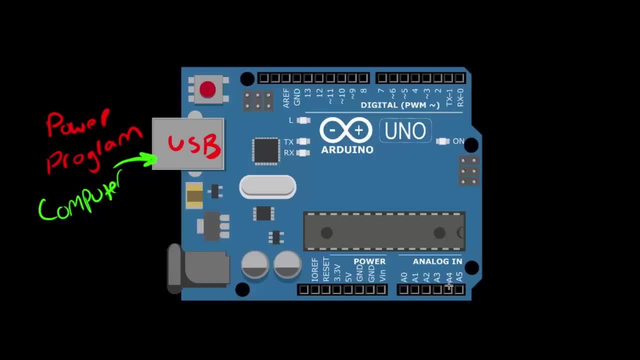 Now there's many different other pins in here. I'm not going to go into detail in this video. We have analog input pins here. Then we have various input and output pins up here, along with PWM pins, and we'll be going into those in a future episode. So in my circuit I want an LED to blink on and off every one. 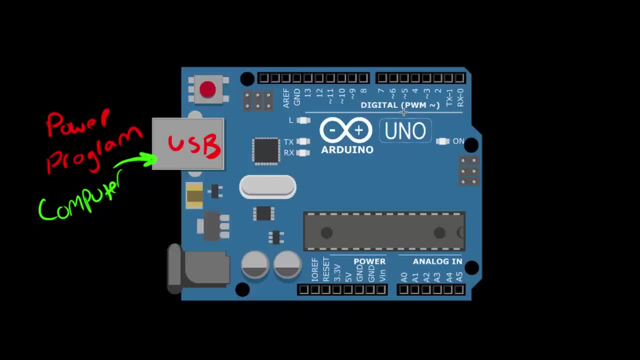 second. I want it to turn on. wait a second, turn off, wait a second, and keep repeating that. So of course we're going to need an LED circuit wired up here. So I'm going to take pin number 8.. And we're 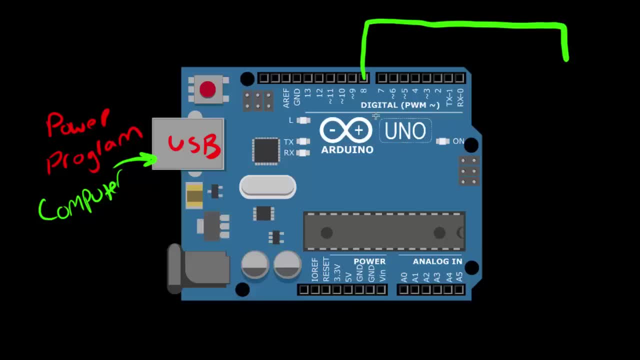 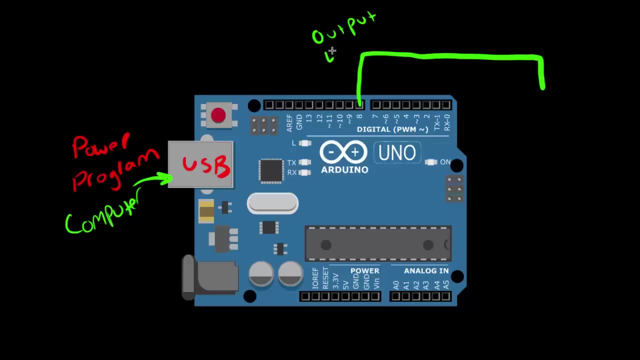 going to say. pin number 8 is: This is our output pin. So this pin is going to be an output, And output basically means we can program it to output either a low signal or a high signal And we can change that signal via our code And we're 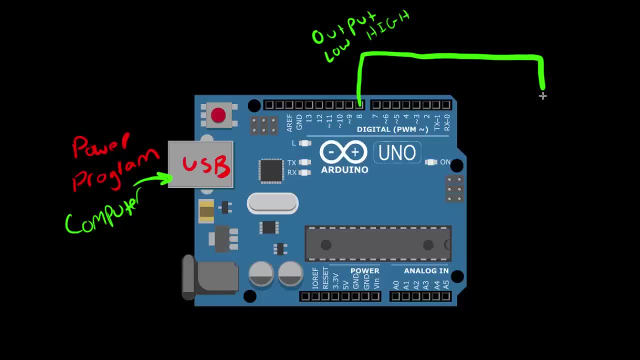 going to see how we do that in just a moment. Anyways, we're going to connect that pin to a resistor, And so that's going to be our resistor. We'll call it R And this is going to be fed in to an LED, So I'll 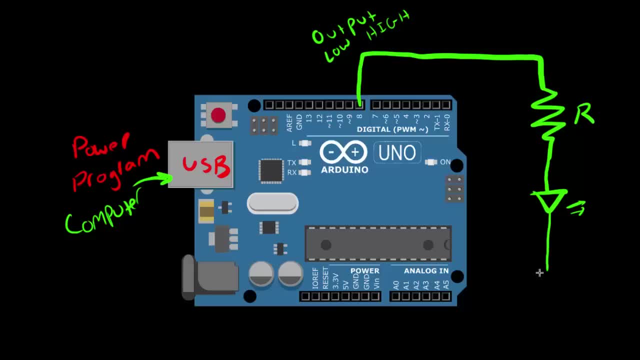 draw my LED symbol here, And after that the LED of course has to be then connected to one of the ground pins on the Arduino Uno. So this is going to be our completed circuit. So if we program it to set pin 8 to low, essentially 0 volts, then our 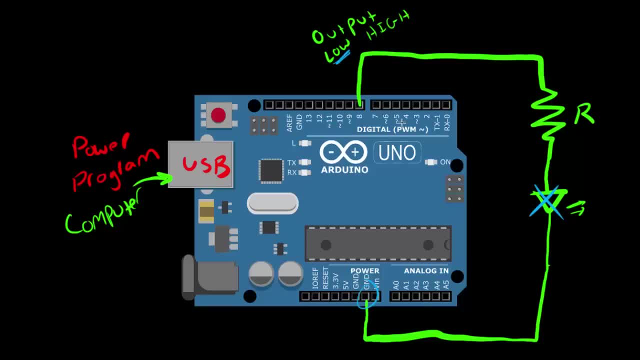 LED is not going to turn on because it's connected to ground here and essentially ground over here. There's no actual high output coming from pin 8.. But if we then wait a second and then program pin 8 to go high or actually have voltage, 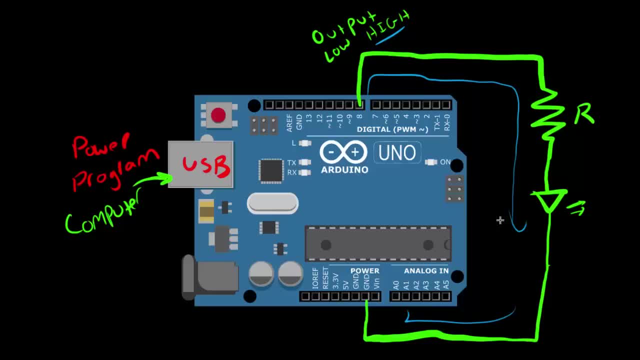 our voltage is going to flow through into the ground and our LED is going to light up, And that's exactly what we want. So we just have to control how often this pin number eight goes high and low. for So, before we begin working on our 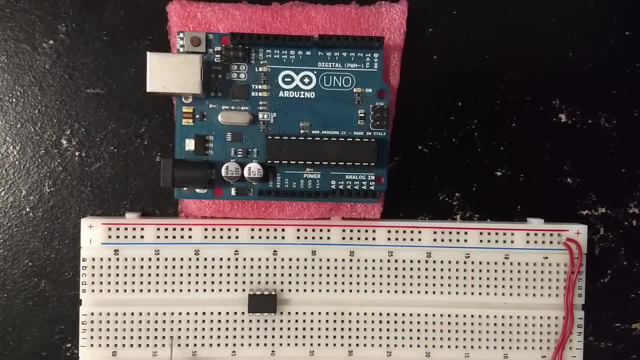 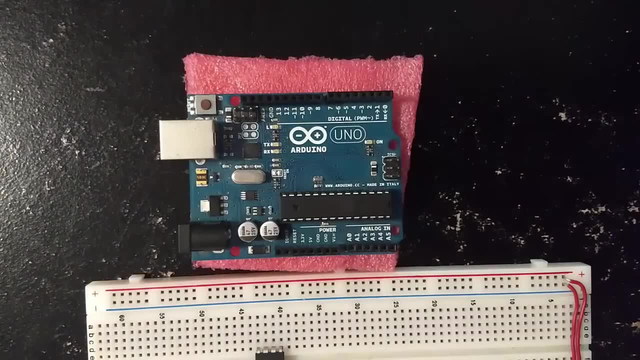 circuit. let's take a look at the Arduino Uno as well as the ATtiny85,, check out their differences and get the Arduino set up for programming. Now here is the Arduino Uno that I have, And the actual microcontroller is just this one. 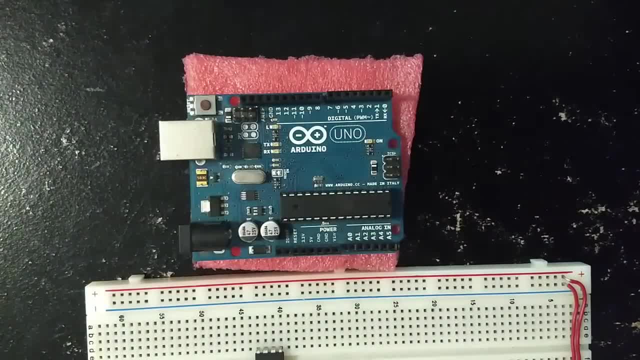 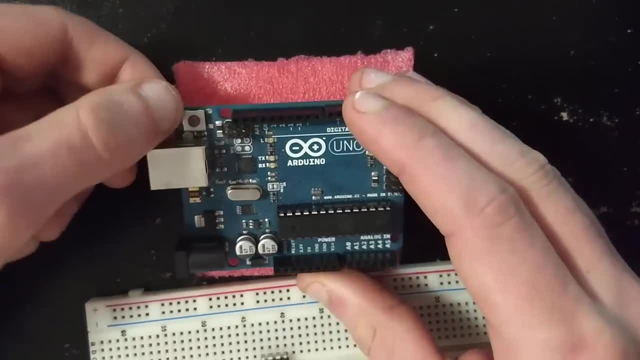 chip here in the board. The rest is all components to a little bit of programming So that it can allow the chip to run properly as well as transfer data from like a USB port on a computer. Now you'll also notice that there's this button in the upper left of the Arduino, And when you push that, that's a reset button. 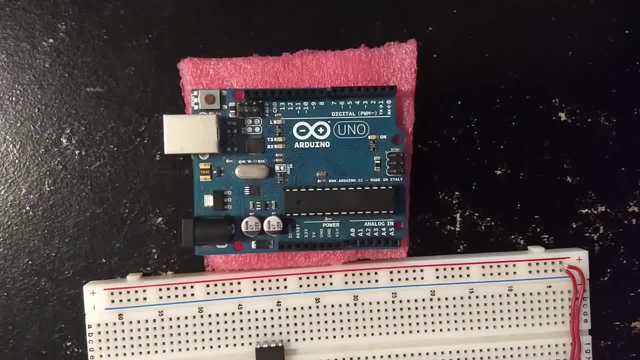 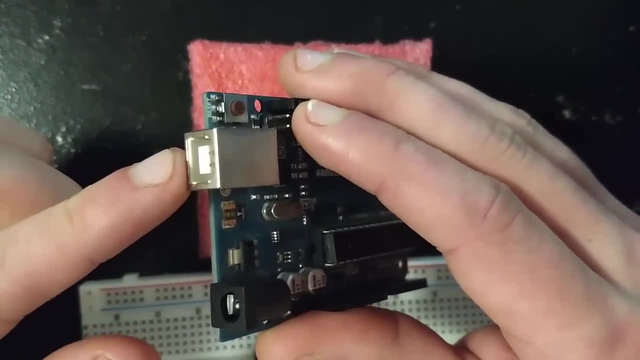 for the Arduino. It'll essentially kind of restart the system for you. Next we can go ahead and see the USB port and the normal power port on the Arduino Uno. Now you'll notice that the USB port here is a USB type B port, So that's very. 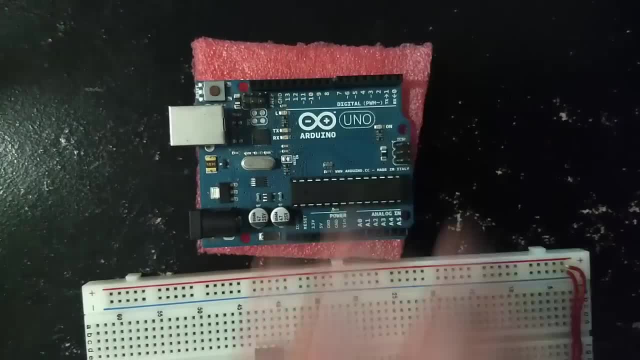 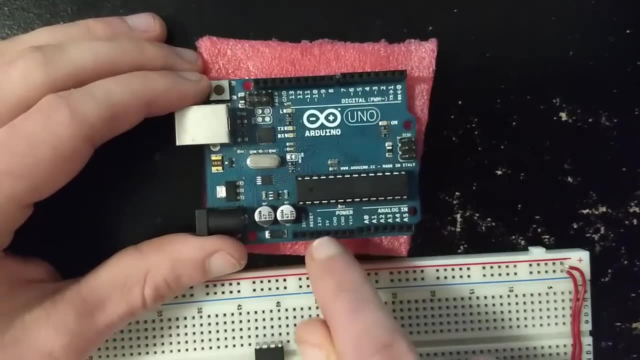 important. So you have to have a USB type B cable, and then your computer can of course have the normal USB port end. So that's the Arduino, and we can see all of the input and output pins everywhere, along with our ground and power pins there. Now let's take a look at this chip here. It looks kind of like. 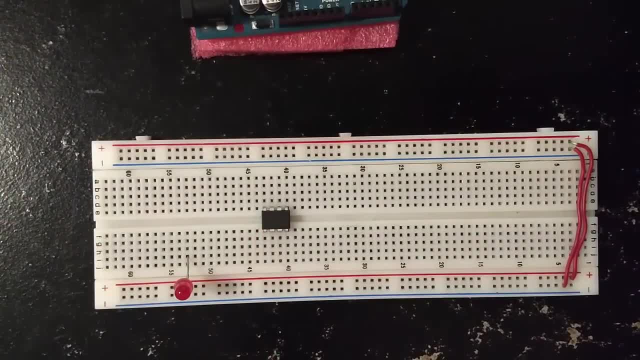 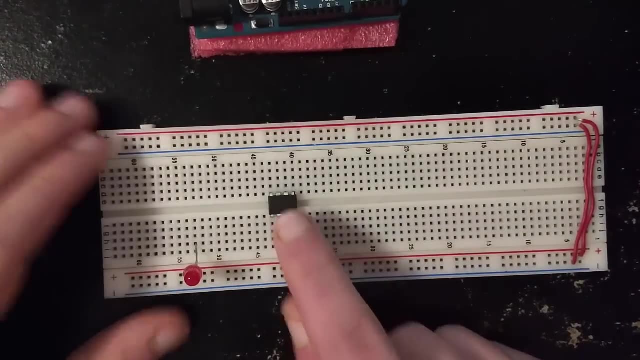 our 555 timer, but instead this is the ATtiny85. So this is much, much different than the Arduino. There's absolutely no way to program this thing using just a USB port. So how would we go about programming something like an ATtiny85? Well, essentially we would wire this ATtiny85 up in. 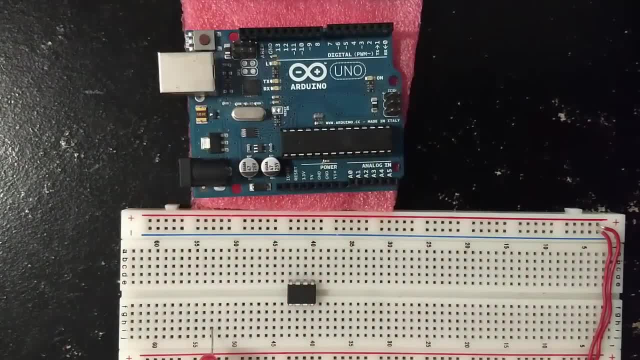 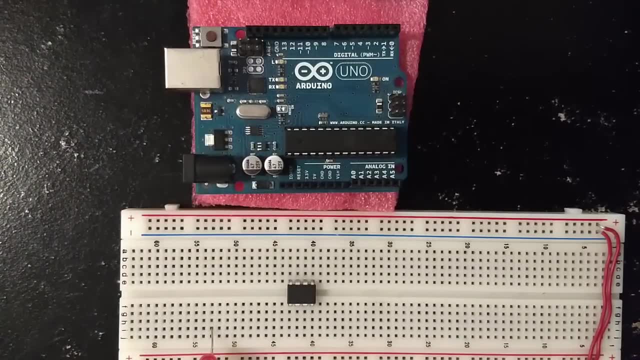 a special configuration using something like an Arduino board here, that we could then upload the code to the Arduino board and then transfer it over to the ATtiny85 using some special software and you know obviously schematics to wire it up properly. Then after that the ATtiny85 would. 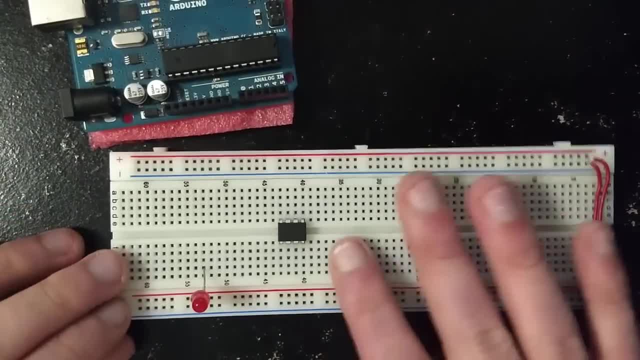 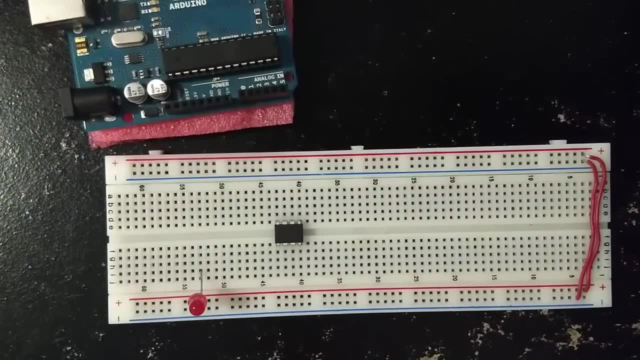 have the code it needs and you can disconnect it from the Arduino Uno and use it as your normal microcontroller chip. Now, if a lot of people want to see this done, I'd be happy to make a video on it, but as of now I don't plan to do so, So let's wire up our circuit here. 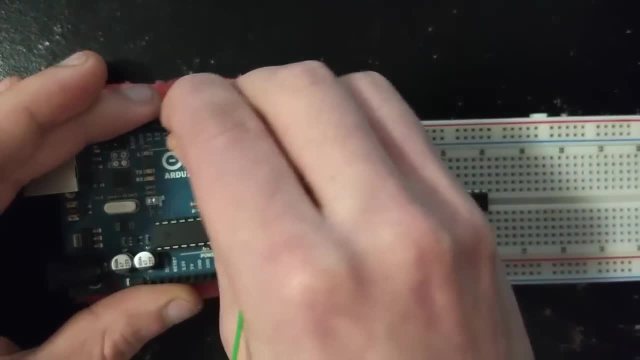 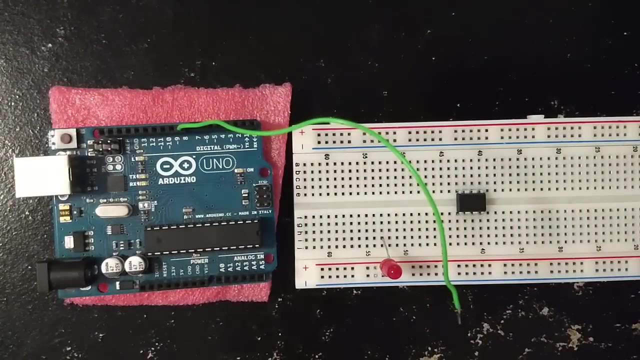 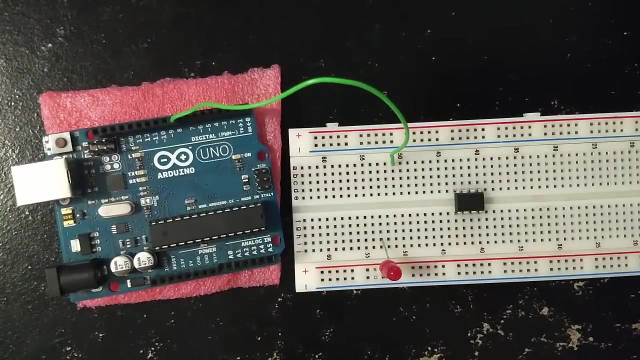 Now, according to my schematic that we just drew, we're going to put a pin, or rather a wire, into pin number 8 here on the Arduino. That's going to be our output pin And I'm just going to plug that into a slot on the breadboard here, And we want this to then go to a resistor, So I'm going to plug in the 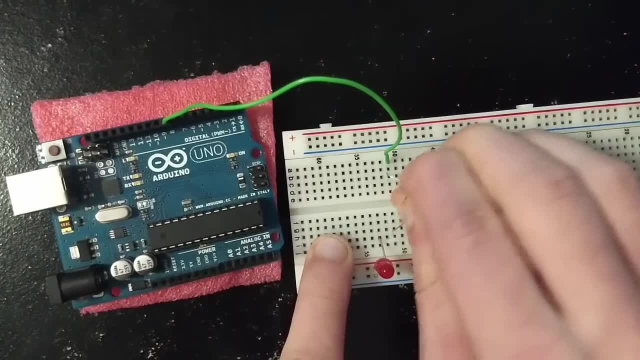 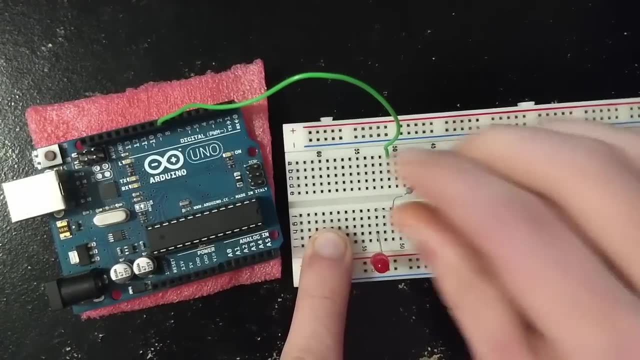 resistor in the same row of the breadboard. Let's make sure that connects here. And then I'm going to plug the other end into the anode, the positive end of our Arduino, And I know I didn't show it, but the other end of the LED is plugged into the ground rail of my. 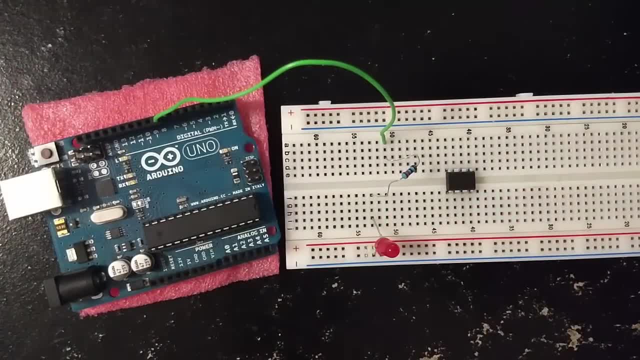 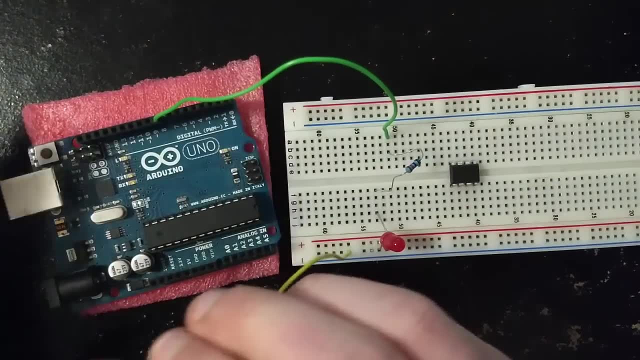 breadboard. So of course we actually have to provide a ground connection to my breadboard. So the final connection is going to be from the ground rail of the breadboard to one of the ground pins on the Arduino Uno. So I'll carefully count to one of the ground pins here, insert it like so and this: 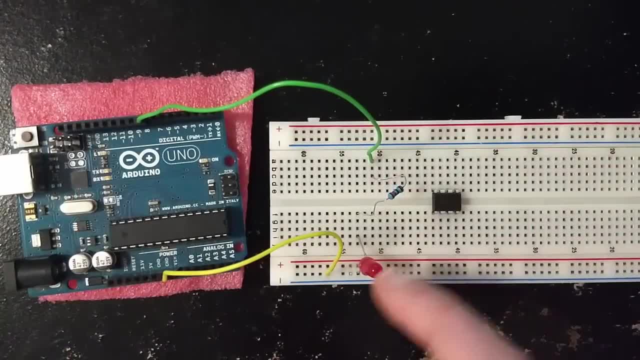 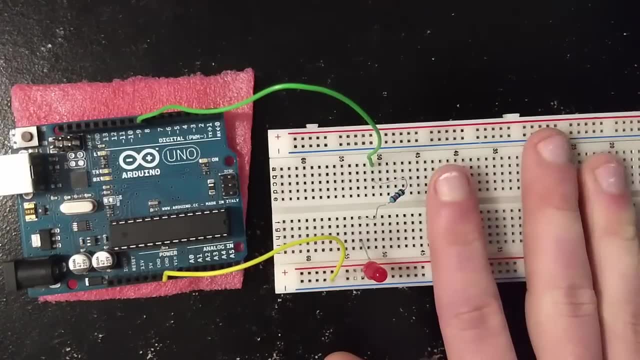 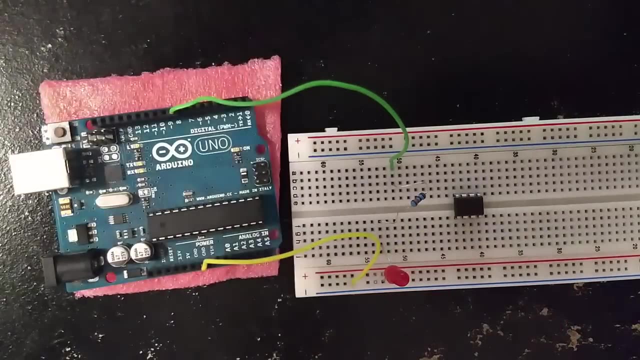 should be our finished setup. We have pin 8 going through a resistor to our LED, to the ground rail, to the ground pin. on the Arduino You can ignore the ATtiny85.. We won't be using that, of course. So now it's all a matter of just programming this. So I have my USB cable here. Let me get it out here. 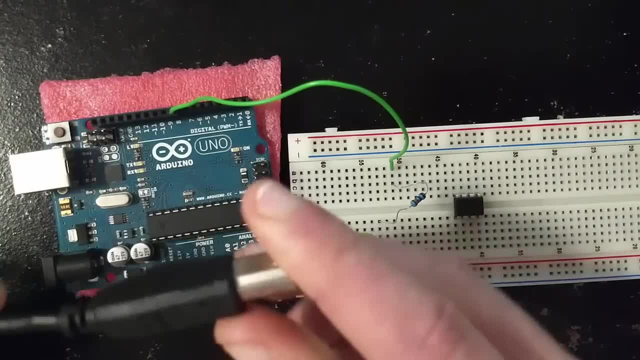 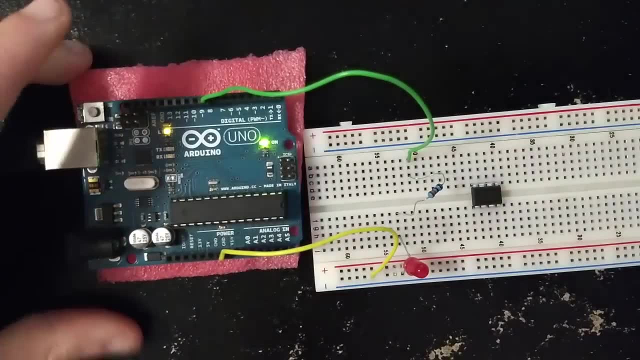 Again, this is a USB type B cable. The other end is just a normal USB cable that I plug into my computer. So that's plugged into my computer. I'll just plug the rest right into the USB port here- You heard my computer there- And the Arduino Uno will light up. Now, of course, nothing's happening because we haven't. 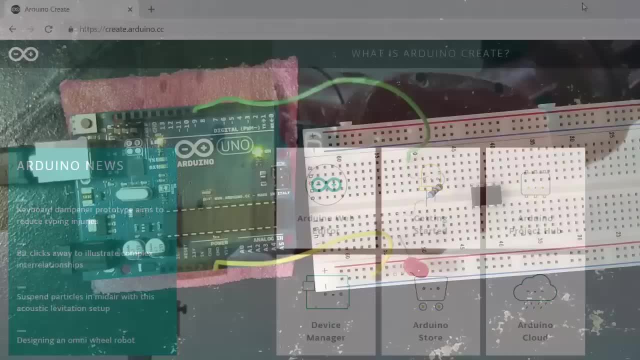 programmed pin 8 through the ground pin on the Arduino, So I'm going to plug that into the ground pin on the Arduino. I'm not going to do anything, So let's go ahead and do that Now. one of the reasons why Arduino is very 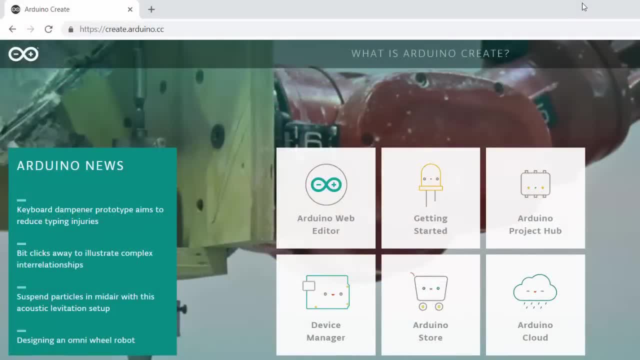 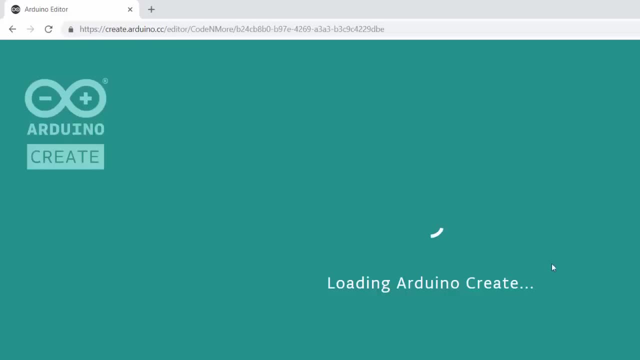 popular is because it's really easy to get set up and it's really easy to upload code to it. I just went to createarduinocc. It's a website And I'm going to click on Arduino Web Editor here. This web editor will. 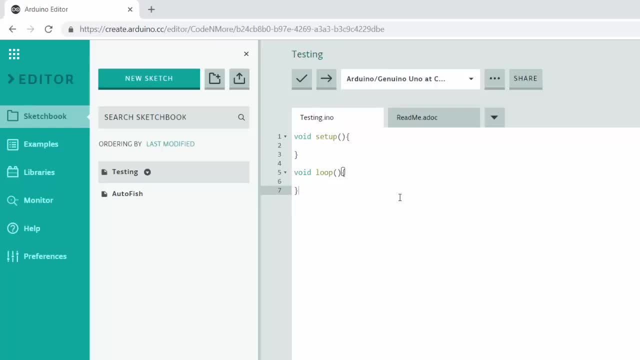 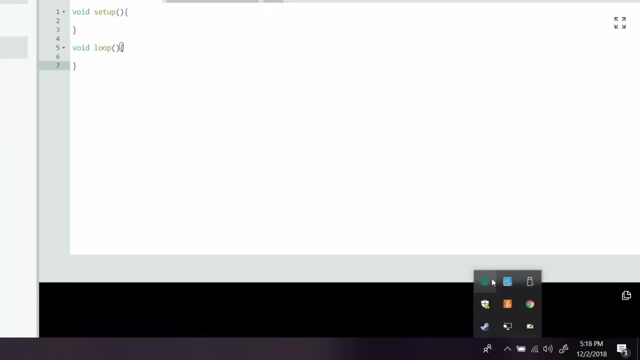 allow us to edit the code for the Arduino and upload it to the Arduino really easily. Now, when you first go to this, it's going to ask you to install a very small program And if we go down to my taskbar here, we see the. 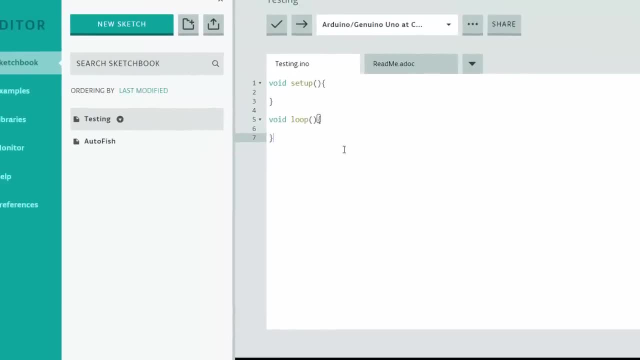 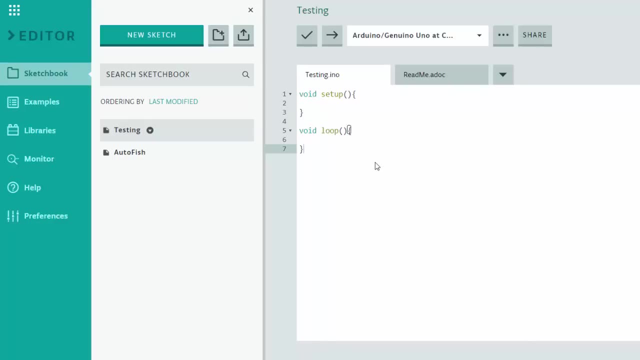 Arduino icon. That's that small program running And that's important because this allows this code editor here to connect to the USB port of the Arduino and actually upload the code for you. So once you get to this point and if you have some trouble, there's a lot of good help in this. 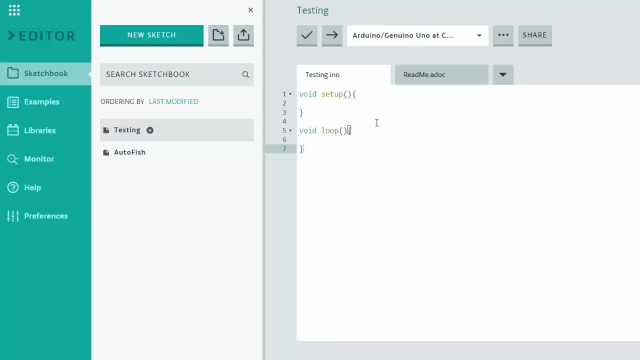 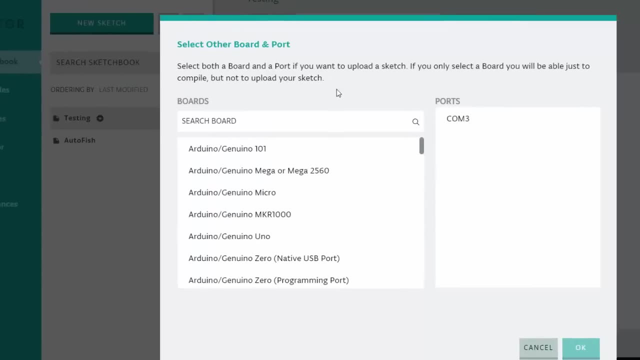 Arduino editor And there's plenty of resources to help you get set up properly. Anyways, once we reach this point, we're going to go up to the device that we want the code to be written for. We're going to go select other board and port And. 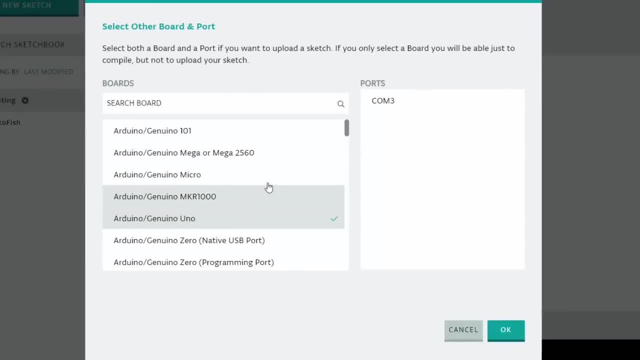 here you would select which board that you're using- in my case an Arduino Uno- And you'd select the COM port that your USB is connected to. In my case it's COM3,. it might very well be a different number for you depending upon what USB port of. 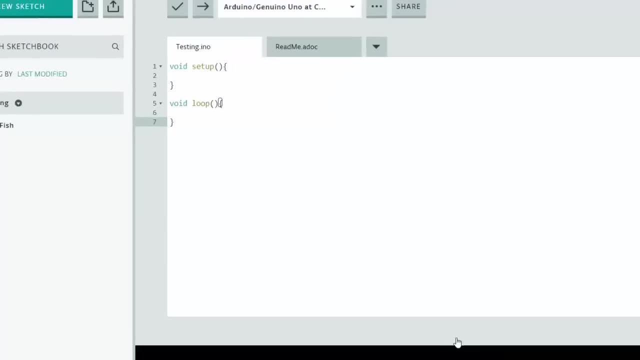 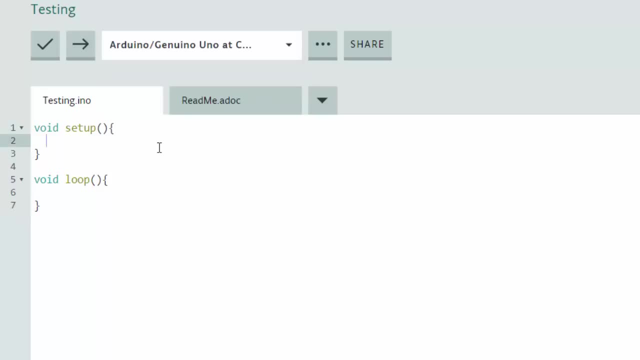 your computer is plugged into the Arduino board. Now I've already done this, So I'm just going to click cancel. But here I have my Arduino Uno at COM3.. That means this web editor here can see my Arduino board and we're ready to get programming. So I just 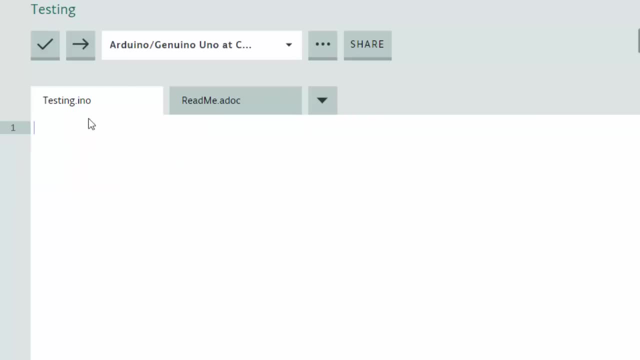 created a blank, a little code document here. It's called testingiono. You can name it whatever you'd like. This is just a code file for Arduino, And we can begin writing our code Now. the first thing that we're going to write is something called void setup. Then we're going to have empty parentheses and then curly. 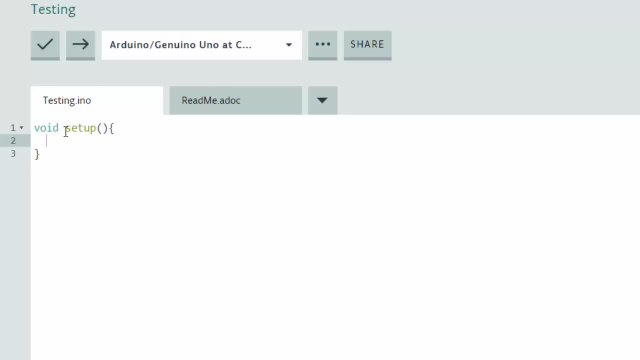 braces. Now, this is very important in Arduino. This is our setup function. Basically, any of the code inside of these curly braces here is going to be run once our Arduino board powers up or once it turns on. So this is the code that gets everything set up for us. Now the 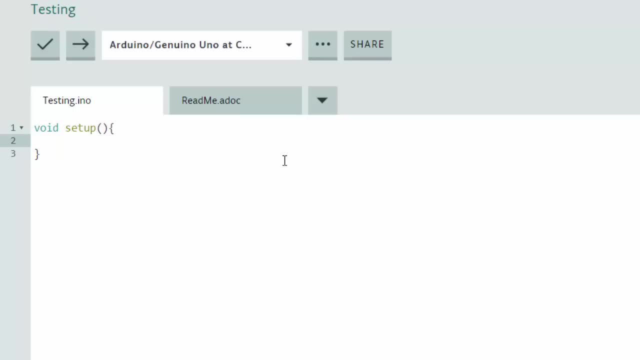 only thing that we need for our circuit in the setup method here is a piece of code that tells Arduino that we want pin number eight to be an output pin. Say hey, we're going to be writing either a low or a high value to pin number eight. Now we have to do this. 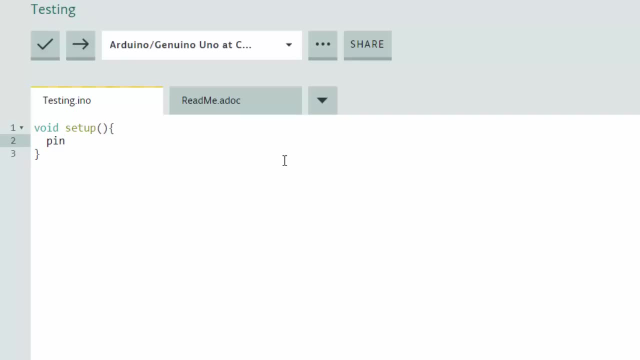 because pins can also be input pins And that's a whole different episode. Anyways, we're going to do pin mode, So we're going to set the mode of a pin and you're going to write the pin number. Now we're using pin number eight, So I'm going to write pin eight there And I'm 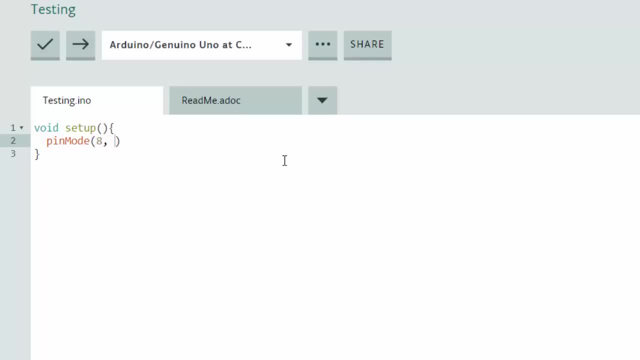 going to put a comma and then we're going to put the mode that we want. In this case we're putting output, because we want pin eight to be an output pin. we're going to write either a low or high value to it. So now Arduino knows that pin number eight is an output pin. we're going to be writing data to it, either a low or a high value. The 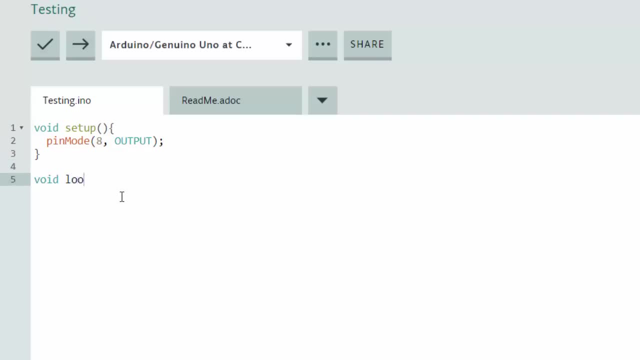 next very important piece of an Arduino program is the loop method. So we're going to write the exact same thing like setup, except it's going to be named loop. Now, this is a little bit different than setup. it's going to run any of the code inside of this loop method after the setup code. 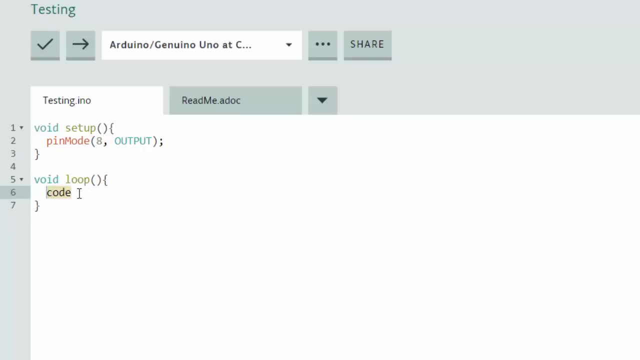 runs, Except once the code completes in this loop method, it's going to do it all over again. it's going to run the code inside of this loop method here over and over, and, over and over again, until your board powers off. So what do we want to do? 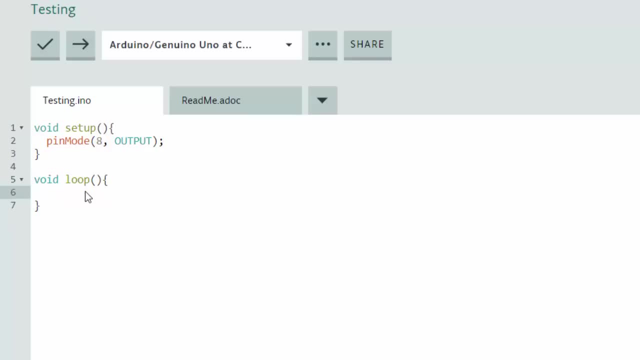 here. Well, we want to turn our LED off, wait for one second, turn the LED on, wait for one second and then repeat that code all over again. So how do we turn the LED off? Well, that's as simple as writing a low value to pin number eight. we want to set pin number eight to zero volts. 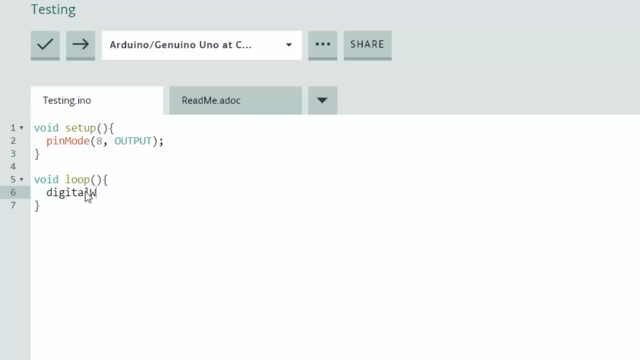 essentially. Now we do that in Arduino by saying digital write, And digital write takes what pin we're writing to. So we're going to write to pin number eight. And then what value do we want to write to pin number eight? Well, we want to turn the LED off, So we have to set pin number eight to a low value. So we're going to type low all capitals. that's going to. 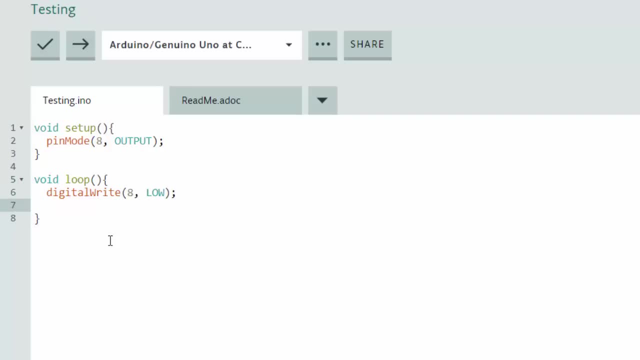 essentially turn pin number eight to output zero volts for us. Next, we want to wait for one second, And we do that in Arduino by saying delay, and then you would think it would be one to be one second, But this delay actually happens in milliseconds, So this would only delay for one millisecond. to delay for one second, we have to type 1000 milliseconds, because there are 1000. 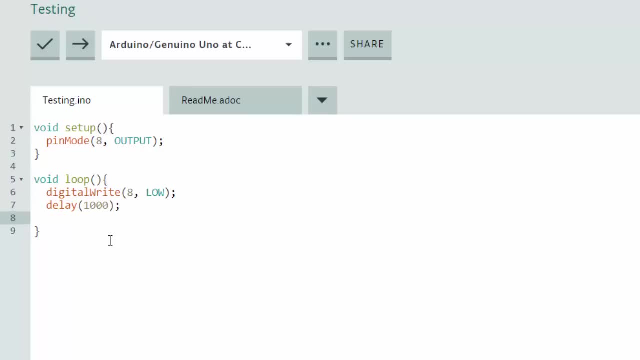 milliseconds in one second. So after we've waited for one second, we then want to turn the LED on. That just means we have to set pin eight to a high voltage now. So we're going to do the same thing digital, right, we're going to write to pin eight, but this time a high value. So we're going to turn voltage on to pin. 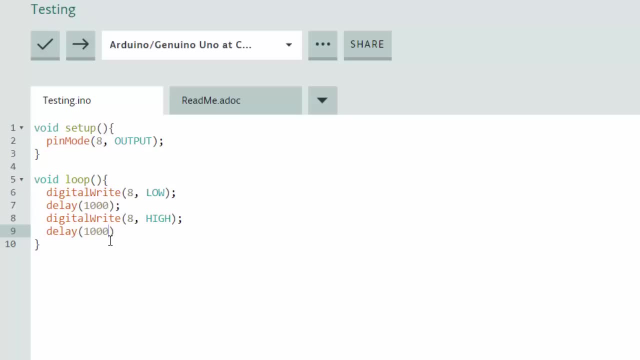 eight. we want to wait for another second. So we're going to delay for 1000 milliseconds. Now, once it reaches here in our code, it's just going to go back to the top of this loop method And it's just going to repeat the code again. So it'll turn the LED off again, wait a second, turn it on, wait a second and then go back up here. 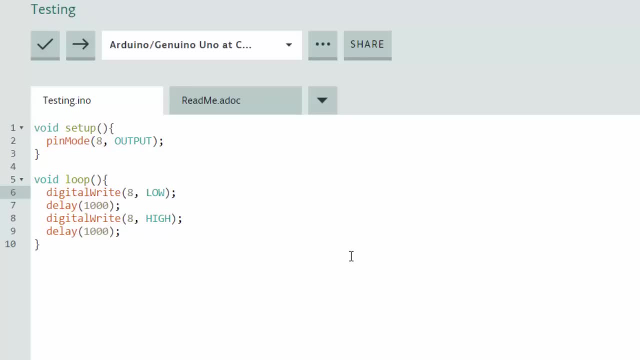 turn it off again And that will never stop until your board powers off. So if you're using this Arduino code editor here, we can click the checkmark up here And that will verify your code to make sure that you don't have any errors in it. So if I would drag up the little console here at the bottom, we can see that it's. 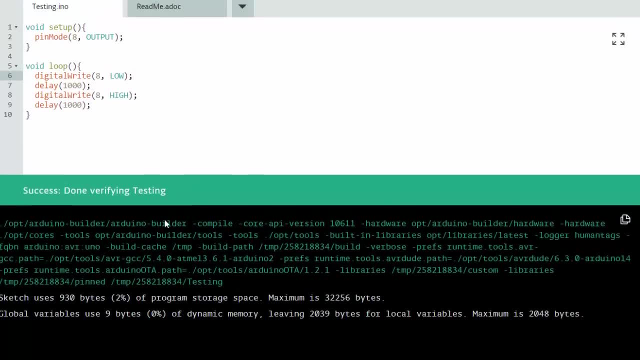 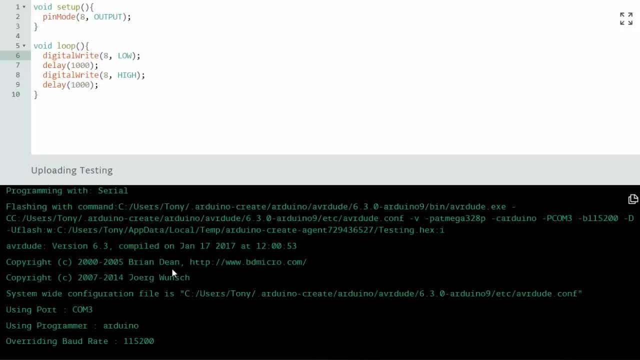 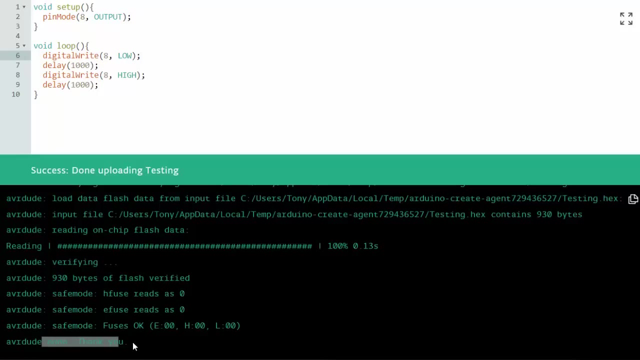 OK, we don't have any error messages. So then we can upload it to our Arduino board. click the upload button right here. it's going to verify your program again and then it's going to try to upload it to your Arduino board through your USB connection. Once it's done, it's going to say done And thank you. 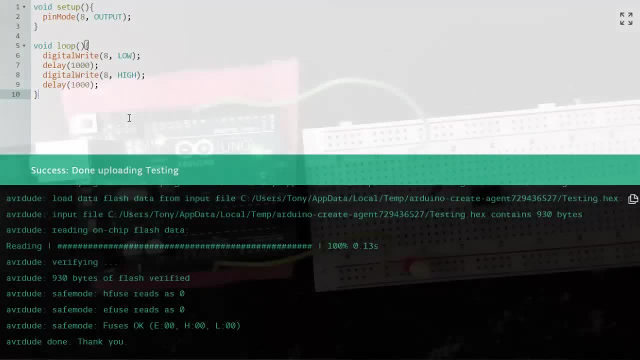 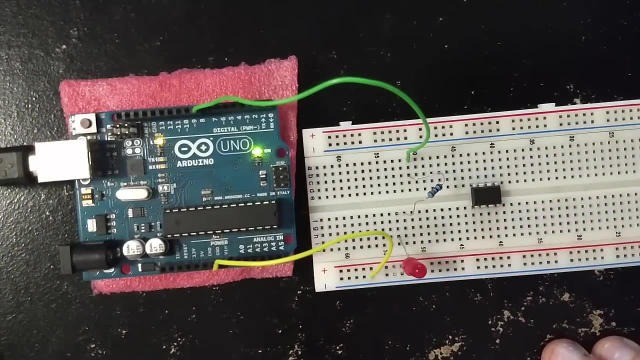 Now let's take a look at our Arduino board and make sure that our code is actually running. So I just uploaded my code to the Arduino And, as you can see right away, once that code was uploaded, we have the LED blinking on and off every one second. 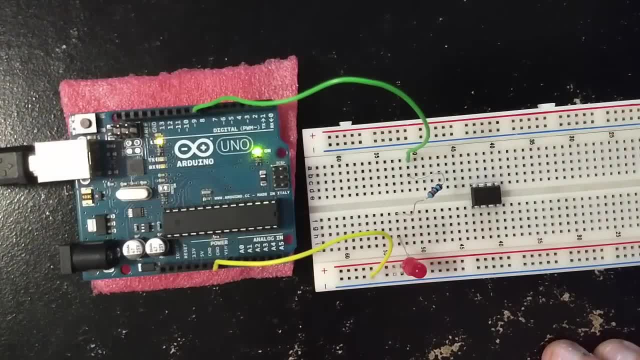 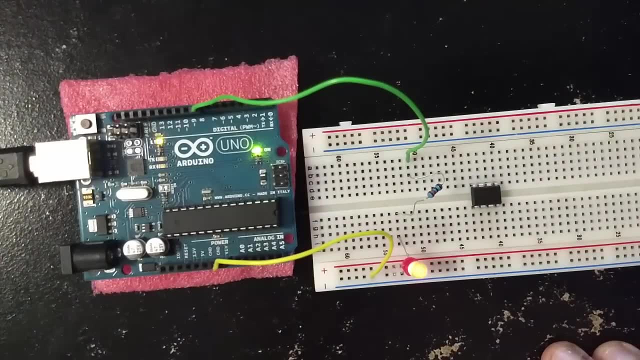 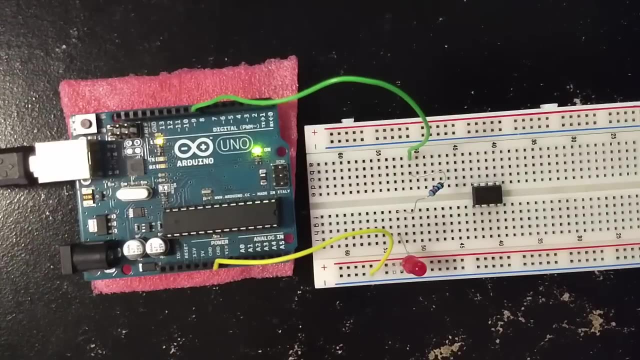 So if we wanted to, we could experiment with this reset pin up here. If we press that button, it'll kind of flicker some lights on the board and it'll reset the system and then restart our programming, blinking once every second. So there we go. That is our completed circuit using Arduino and Arduino code. These things are extremely fun to play around with. You can make ridiculous amounts of projects with things like the Arduino, So if you're into this type of stuff, I highly recommend getting one and experimenting with it. Thank you all so much for watching. And I'll see you guys in the next episode. 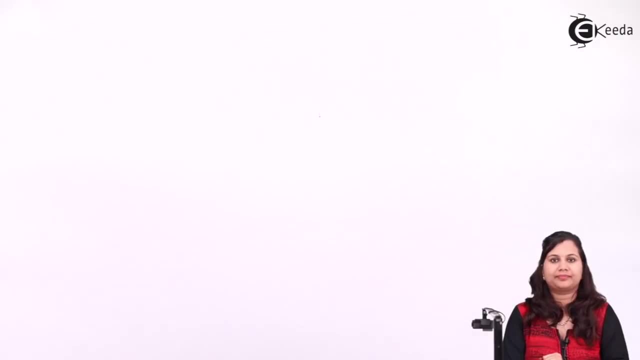 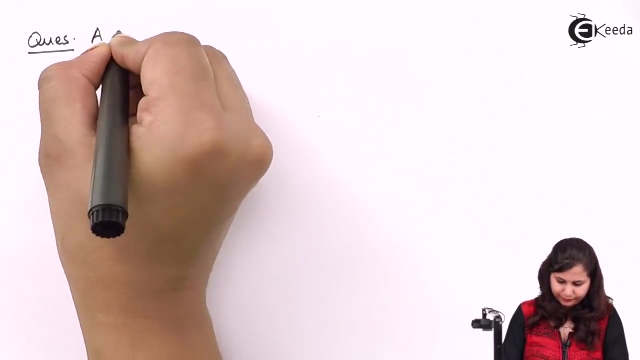 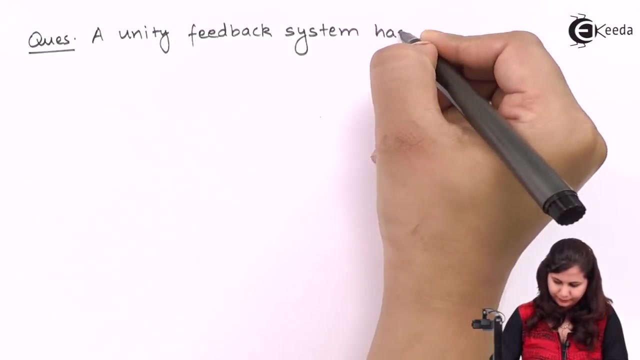 Hello, friends, in this video we are going to solve a problem on how to draw the Nyquist plot of a system whose transfer function is given to us. So let's take a problem. Hello friends, in this video we are going to solve a problem on how to draw the Nyquist plot of a system whose transfer function is given to us. So let's take a problem. 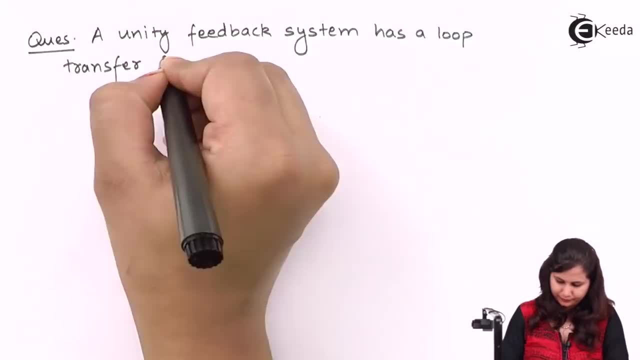 Hello, friends, in this video we are going to solve a problem on how to draw the Nyquist plot of a system whose transfer function is given to us. So let's take a problem. Hello friends, in this video we are going to solve a problem on how to draw the Nyquist plot of a system whose transfer function is given to us. So let's take a problem. 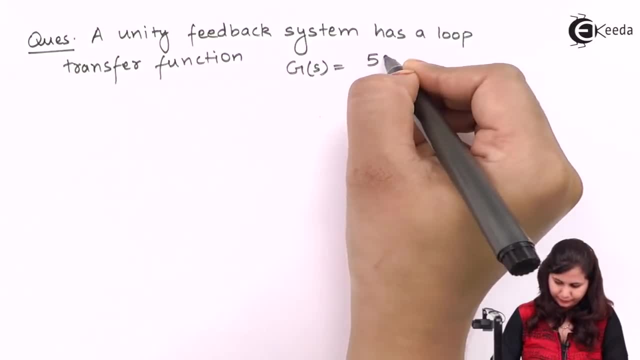